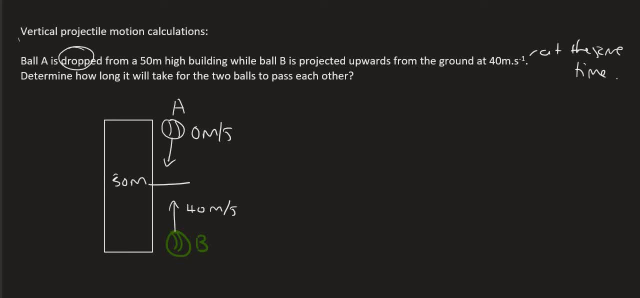 the key thing to remember is that the ball b is projected upwards from the ground at 40 meters per second, so that means that the two balls are not going to travel 25 meters and 25 meters. but what we do know is the following: let's assume that ball b manages to travel 30 meters before. 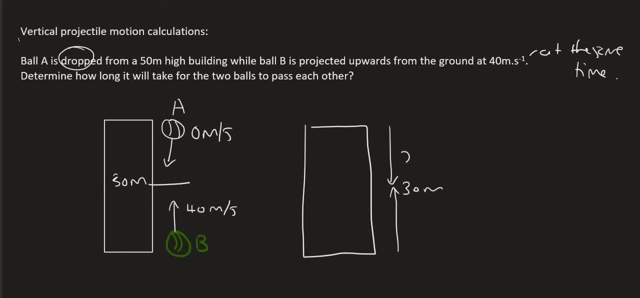 they go past each other. well then, that means ball a would have to have gone 20 meters, so that the total is always going to be 50. so what we can say is that the displacement, or no, actually the distance that ball a travels, plus the distance that ball b. 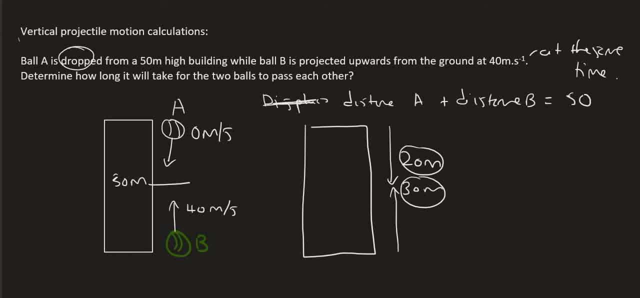 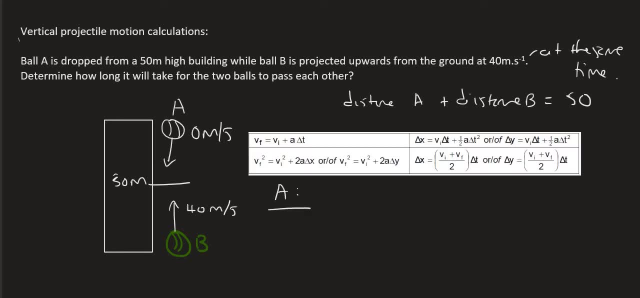 travels should give us 50.. that's the key concept we need to know. so let's bring out our formulas, okay? so let's do ball a first. now we're looking for the displacement, okay. so we don't know what that is, but we know the initial velocity of a and we know it's acceleration, so what we can use is 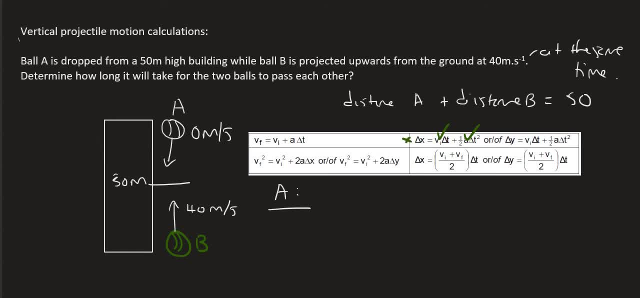 we can use this formula over here and for ball a, i'm going to choose downwards as positive, because then i know that if i choose downwards as positive, is ball a going to end up below the position that it started at. yes, it is, and so i know that the displacement answer is going to be positive. so that's good. so we're going to say: 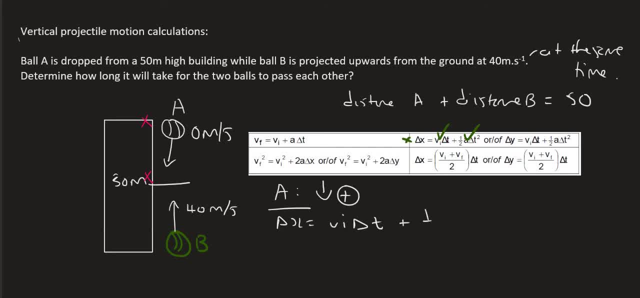 change in x equals to v, initial change in time plus a half a change in time squared. and so the initial velocity is zero, gravity is positive 9.8, because it's traveling downwards and gravity acts downwards, and the time we don't know. then i'm going to do the same for b, but i know that b is going to end up higher than where it. 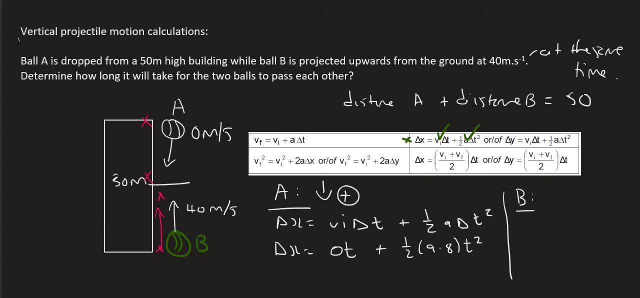 starts, and i want that displacement value to be a positive, so that when i add them together i get 50.. okay, you want them both to both be positive. so for b i'm going to choose upwards as positive, and so i'm going to use the same formula. so let me just write this out and so: 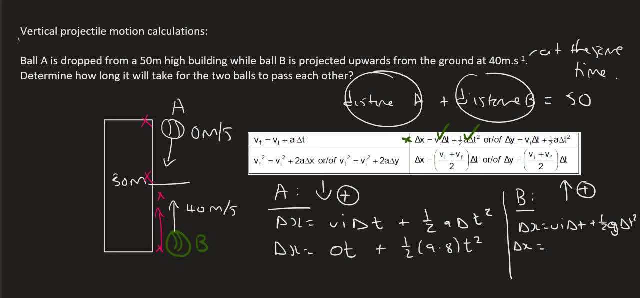 the initial velocity, velocity of b is 40 and it's going upwards, and so we can keep that as positive. we chose up as positive, and so then then gravity will have to be negative because we're choosing upwards as positive, t squared, and so i know that this is going to give me a positive answer, because 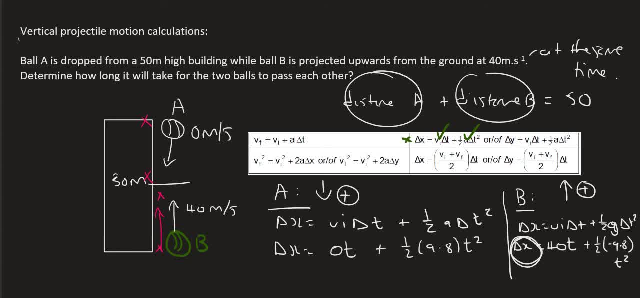 it's: ball b is ending up higher than where it started, and i know that this formula is going to give me a positive answer, because ball b is going to- i mean boy is going to- end up lower than where it started. if i had chosen positive- i mean upwards is positive for both of them. 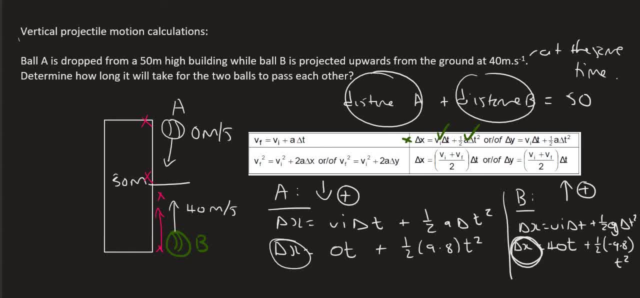 then bore a's answer wouldn't, it would be a negative, and so ball a would be like minus 20. and so then the distance for b to try make 50, it means that the distance of b would have to be 70. now that can't happen because the building's only 50 meters tall. so we want to know both of the. 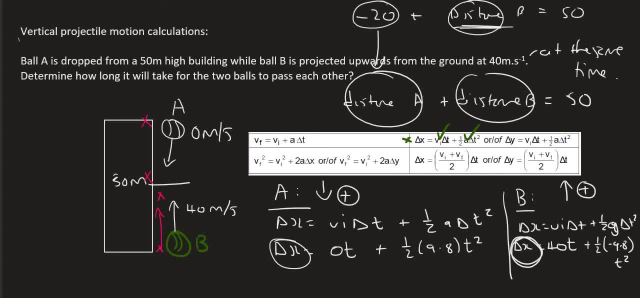 positive. we want both of their distances or their displacements to be positive, and so you have to be clever with your direction choice for each ball. so this is going to be for a and this is going to be for b, so then what we can say is that the displacement for a plus the displacement for b. 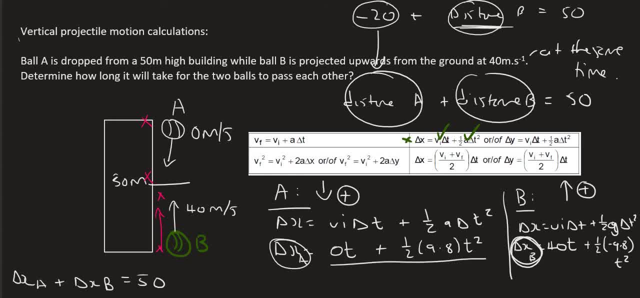 should give us 50.. so i'm just going to fill these formulas in. so that's going to be therefore, 0 t plus a half times 9.8 t squared plus. now i'm going to do ball b, which is 40 t plus a half times. 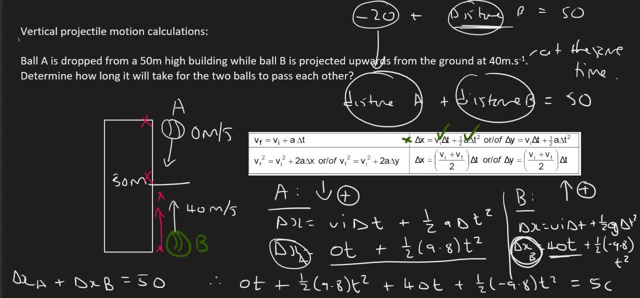 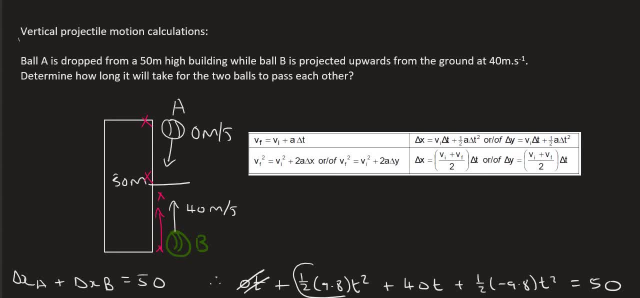 minus 9.8 t squared should give us 50. now it just becomes a matter of solving this equation. so this part here is 0, this part here becomes 4.9 t squared plus 40 t. but then this part is minus 4.9 t squared and that should equal 50. so what's nice is that that part and that part cancels. 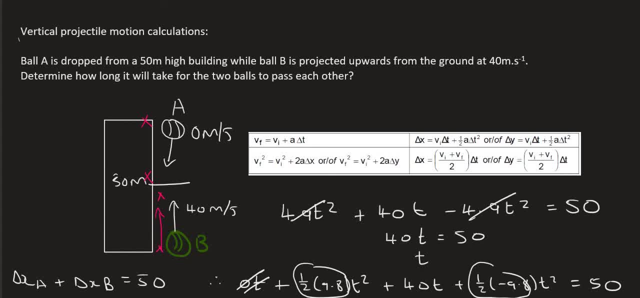 and so we end up with 40. t equals to 50, and so if you had to go and divide, you'd end up with: t is equal to 1.2 seconds. so it will take 1.2 seconds until the two balls go past each other. 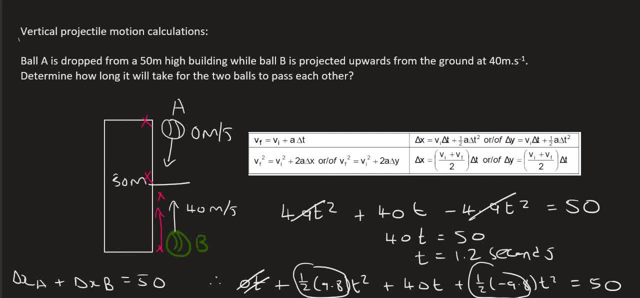 so, please, if this video didn't make sense, please watch it once, or maybe another two more times until it makes sense. as i said, it is in many exams that i've seen. the important thing is just to choose a individual choice of direction for each one, because, as i said, if we chose upwards, as